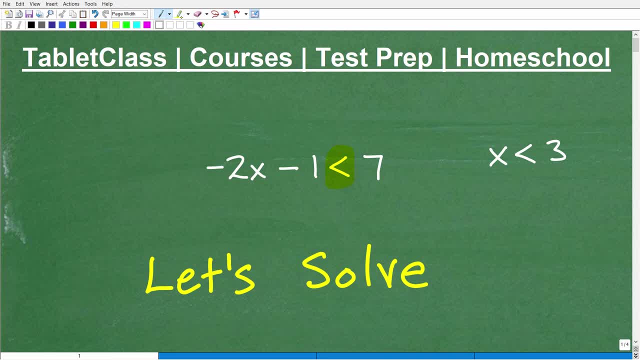 No, X is less than three. So what is X? What is the answer to this problem? Okay, well, if you said two, okay, X must be two because two is less than three. Well, that's pretty good, That's a pretty good answer. 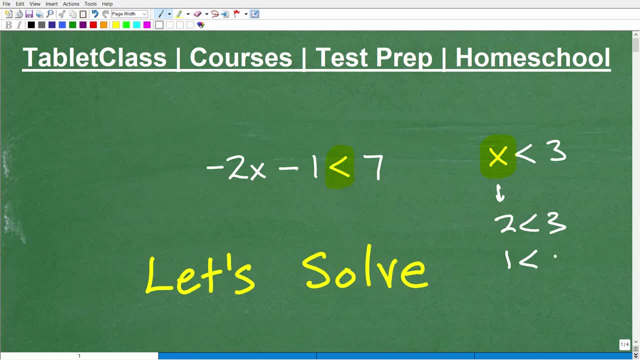 However, are there any more answers? Well, yeah, one is less than three. Zero is less than three. Matter of fact, 2.87 is less than three. So how many answers can X be Okay? well, X can actually be an infinite amount of numbers. All these numbers that are less than three are actually a huge amount, an infinite amount. So that's why, when we express our solutions with inequalities, we often use graphs. 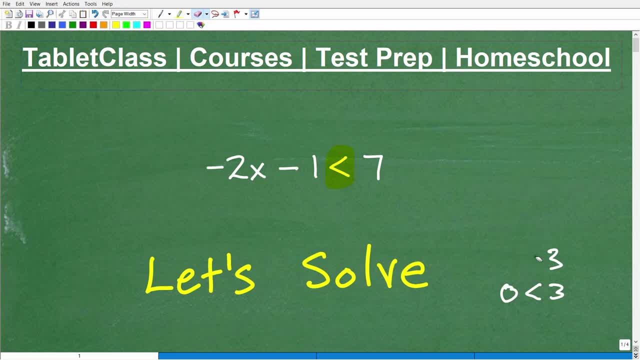 And it's not like an optional thing. You need to understand it. But this was a quick, just you know- review of real basic concepts with inequalities, And it's certainly something you need to understand completely if you expect to be successful in algebra, which I know you can be All right. so we're going to get to this problem and exactly what to do with it and the skills you need before you even attempt this problem, in just one second. But first let me quickly introduce myself. My name is John. I'm the founder of Taba Class Math. 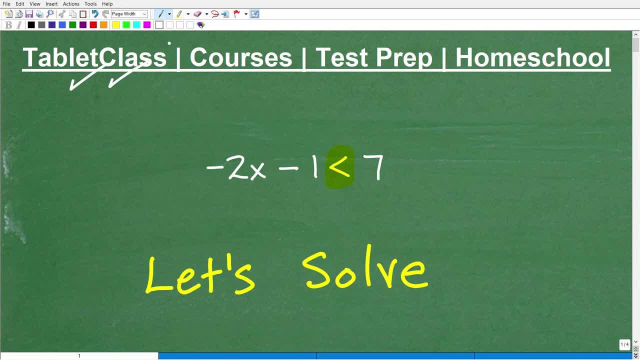 I'm also a middle and high school math teacher And I just want to tell you very briefly about my math help program. You can find a link to it in the description of this video. But basically I have 100 plus different math courses, ranging from pre-algebra to pre-calculus and everything in between. I also have a ton of test prep courses. So if you're taking any exam that has math on it- examples would be the GED, SAT, HiSET, ACCUPLACER, teacher certification exam, ASVAB- You kind of get the idea. I can go on and on and on If you're taking any exam that has math on it. I'm also a middle and high school math teacher And I just want to tell you very briefly about my math help program. You can find a link to it in the description of this video. But basically I have 100 plus different math courses ranging from pre-algebra to pre-calculus and everything in between. I also have a ton of test prep courses, So 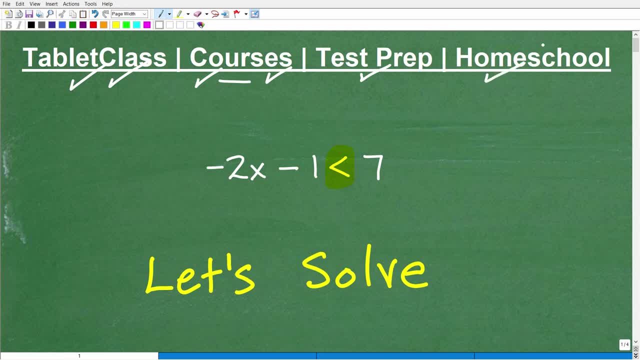 if you're taking any exam that has math on it, I can help you prepare. I also have a great homeschool program. So if you homeschool, you definitely want to check out what I have to offer. Then obviously, help those who are having a tough time in your current math courses. Now, if you are a student and your notes are anything less than outstanding, you need to work on your notes. I've been teaching math for decades. I'm telling you right now, most students don't realize how important their notes are. Take great notes and things will get better for you in mathematics and probably all your other subjects as well. By the way, I have a 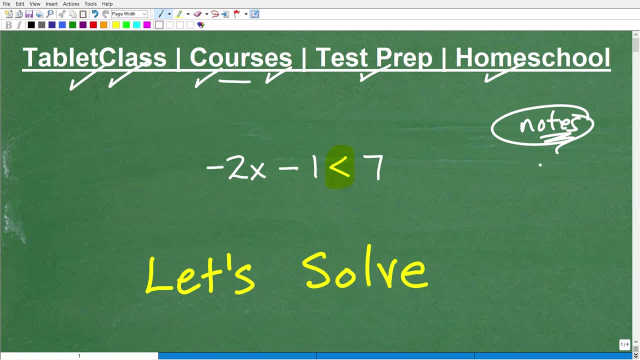 notes, math notes, and I'm going to leave links to all my different math notes in the description of this video if you want to check those out, Okay, so here is our lovely problem. Now, if you think you can solve this problem, okay, solve it and graph it. then you know, turn this into a pop quiz, pause video. It should take you all of about- oh, I don't know- 45 seconds at most to do this, if you know what you're doing. But let's talk about a couple things here. Before you start this problem, you need to know how to solve. 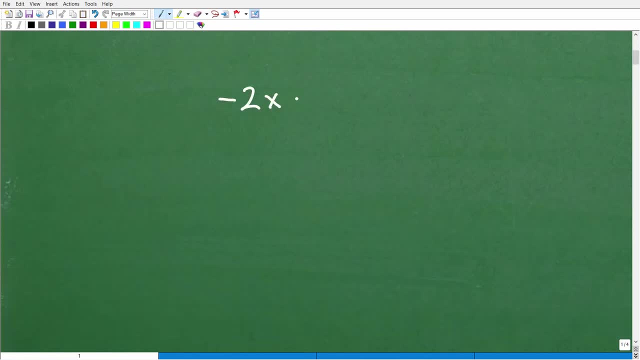 basic equations, So you would need to know how to solve something like this, Okay, so how do I solve this problem? Can you solve this equation Now? if you can't solve this equation, you're going to have a difficult time with this inequality. So the first step when you're learning how to work with inequalities is make sure you know how to solve algebraic equations. Okay, so a lot of students still struggle with inequalities because they really, you know, had a tough time with you know they really still struggle with equations. So let's just quickly review. 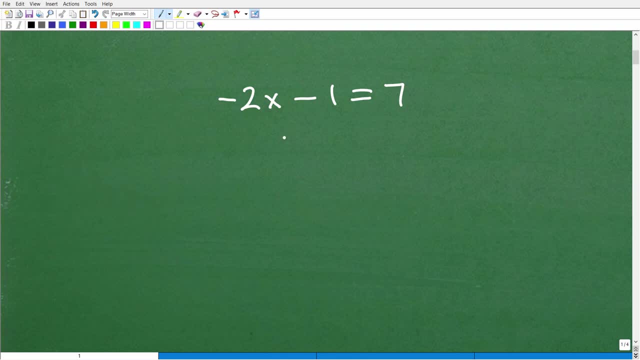 This particular problem. Okay, so how do I solve for x? Well, what I'm going to do is I'm going to add one to both sides of the equation. Okay, I don't want to turn this into a whole video on solving equations, But let's just do go ahead and review this. So negative two x plus zero is going to be negative. two x negative one plus one is zero. that goes away. Of course. I'm adding one to both sides of the equation. That's what I need to do. Seven plus one is eight. So now I got this nice little one step equation. negative two x is equal to. 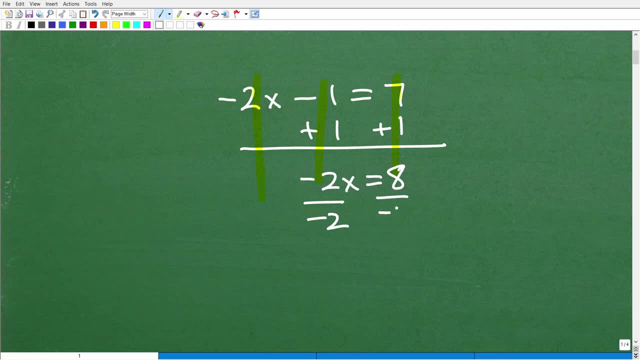 eight. So to solve for x, I got to divide both sides of the equation by negative two. So x is equal to negative four. Now, if you're able to do this problem on your own- you totally understand that- then I must give you a nice little happy face, with a few check marks and a couple stars, just to make you feel a little extra special. Okay, so nice job, right? So if you know how to solve these basic equations, then you should have no problem with inequalities. However, there is a couple different twists, And what we're talking about here is something called 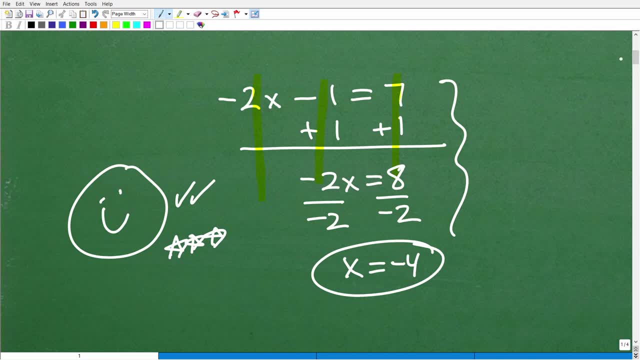 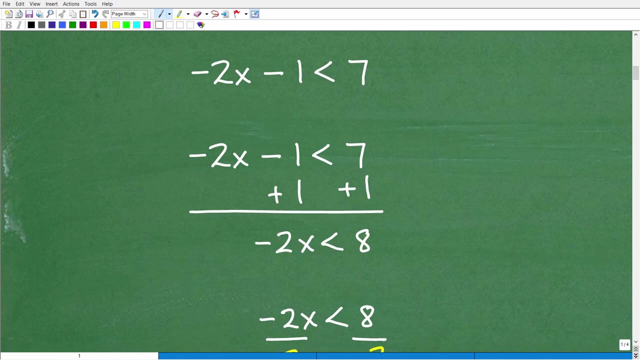 linear inequalities, or there's an additional topic with inequality is called compound inequalities. then we can graph inequalities, we can have systems of inequalities, and the fun just continues. But let's just focus on this problem here, All right. so what we're going to do is we're going to kind of think of our little inequality symbol temporarily in our brain as an equal symbol. we're going to kind of treat it as an equal symbol. we're going to follow the same steps. 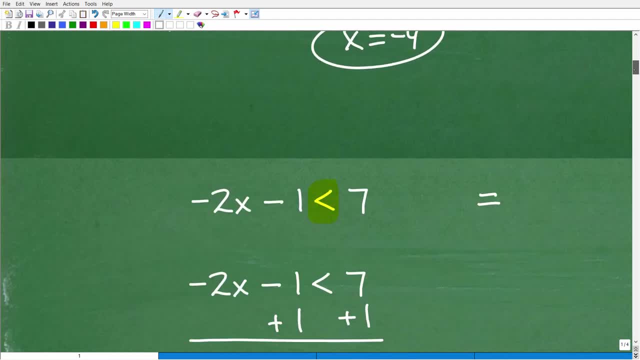 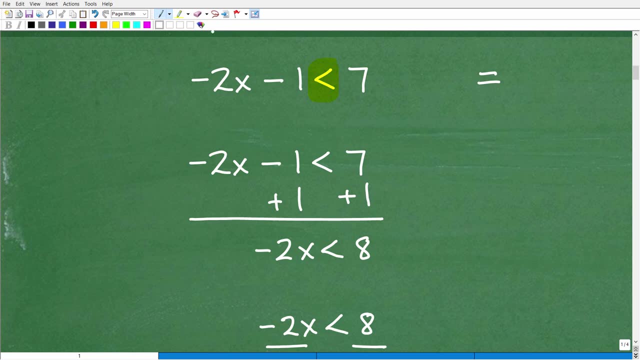 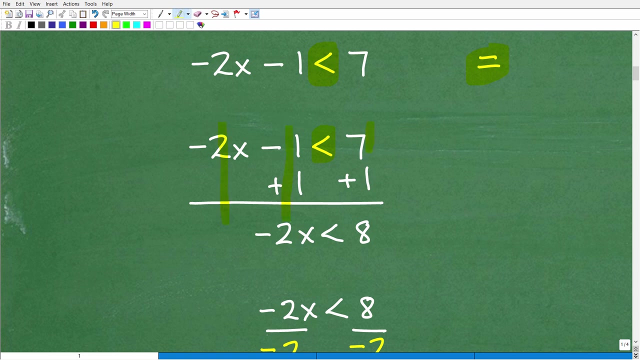 That we just did right over here, Okay. However, we got to be paying attention because there were some things that that affect the way this problem turns out, All right. So, with that being said, here is our inequality symbol. we're going to kind of think of it as an equal sign, more or less. So it's the same steps as the previous problem. I'm going to add one to both sides of the inequality, All right, so I'm adding down like: so. So I get negative two x plus zero is just negative two x. the one. this negative one goes. 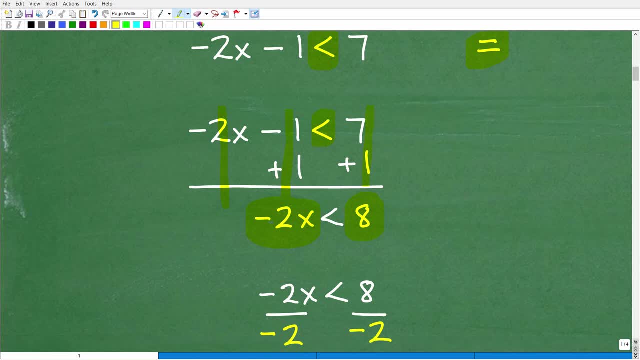 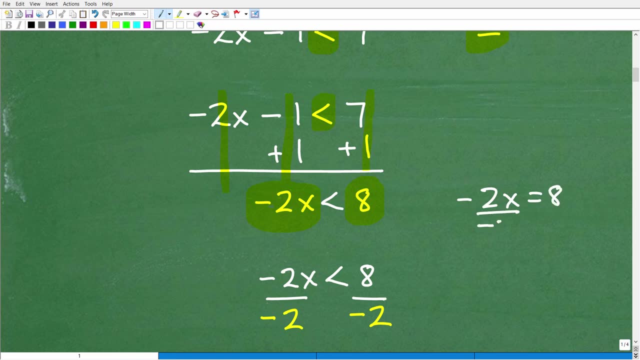 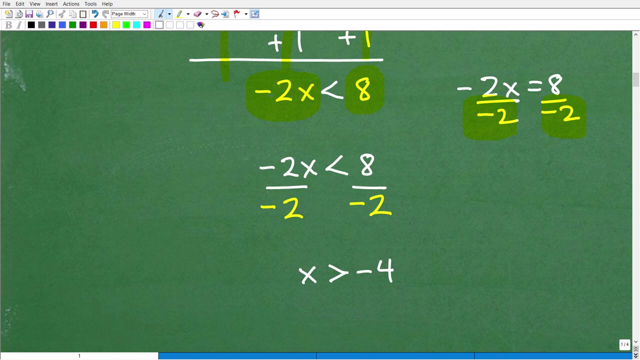 away and I have: seven plus one is equal to eight. All right, so just thinking of this as if this was negative two, x is equal to eight. I would just divide both sides equation by negative two And I would have my answer. But what am I doing in this step? I'm dividing by a negative number. Okay, now, this is where you you know. this is why you have to take notes, because there's all these little details here. Anytime you divide by a negative number, okay, when we're talking about 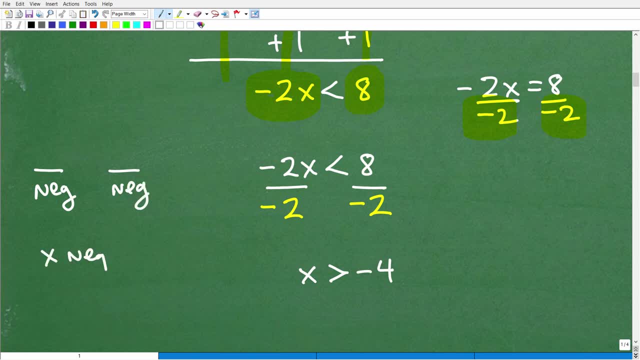 inequalities only, or you multiply both sides of the equation by a negative number, then you must do the following: This is critical, critical, critical. you want to pay attention to me? Okay, So here this is less than. now notice what happens to the inequality symbol: it flips, it reverses. Okay, less than is going to become greater than. if I had greater than, it would become less than. So, anytime not. when you divide by a number, by a negative value. 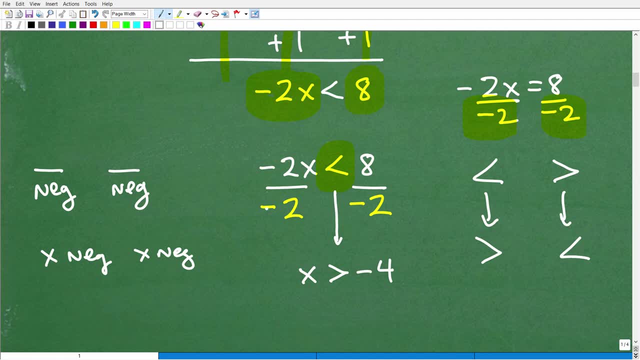 okay. so if you're multiplying or dividing both sides of the inequality by a negative value, you reverse the inequality symbol. So when I do that, I end up with: x is greater than negative four, because eight divided by negative two is negative four. That is the solution. Okay, Now, if you got that right, then I must give you my awesome 1983. Crazy Mohawk. Okay, yeah, we used to. I don't know what it was. back in the 80s, We liked crazy hair And we also liked hairspray. 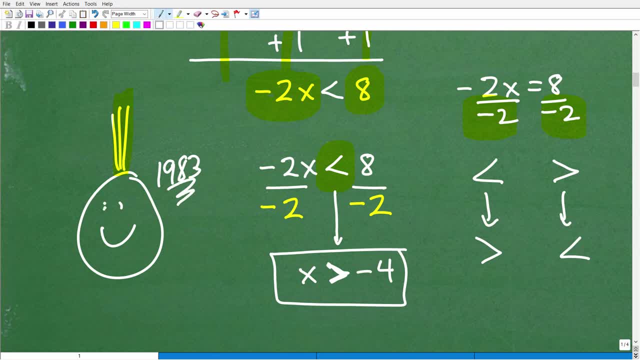 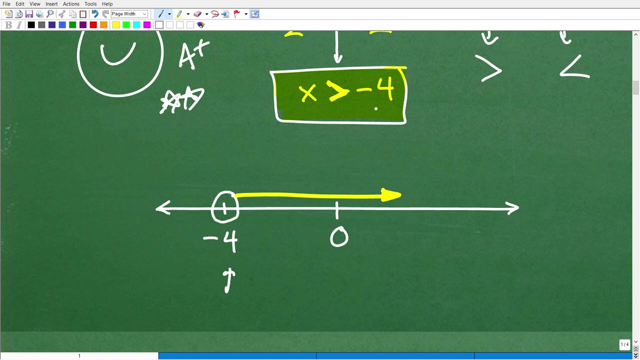 I'm pretty sure that wasn't the safest haircut to be walking around with, But anyways, nice job. I will actually give you an A plus and a couple of stars. However, we're not done Because we want to represent this right here graphically: Okay, x is greater than negative four. Okay, so this is what your teacher would expect you to have. We have a number line graph. Here's zero, Here's negative four. Okay, notice, I'm putting this down right here on a number line. Then you, because this right here is: 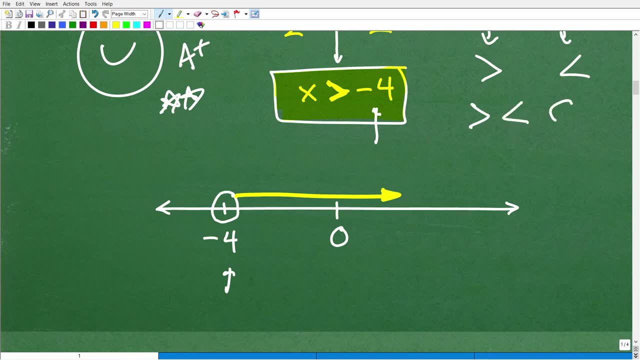 greater than so, greater than and less than, you're going to use what we call an open circle. If it's greater, greater than or equal to, less than or equal to, you're going to fill in the circle. So this doesn't is not an equal to, it's just greater than. so I'm going to have an open circle, which means that negative four is not an answer. Negative four is not greater than negative four. Negative four is greater than or equal to negative four. That's when you fill that in Again. I have a ton of other videos on this in my pre algebra and algebra playlist on inequalities.